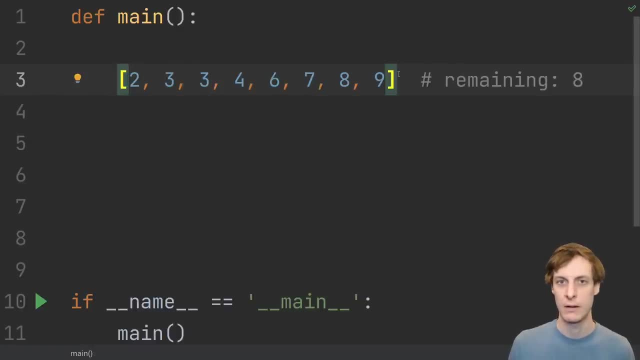 Hello and welcome. I'm James Murphy, and today we're talking about binary search. Binary search, also called bisection search, is an algorithm for finding an element quickly in a sorted array. Suppose we're trying to find 7 in this array. Is it in the left half or the right half? 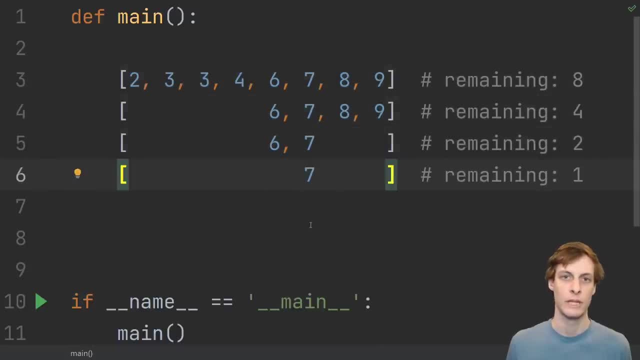 The right half And then repeat. Finally, there's just one element left. That's our 7.. Even though it's one of the first algorithms that one learns, it's also extremely important. Analyzing binary search is often the branching point for studying things like time complexities. 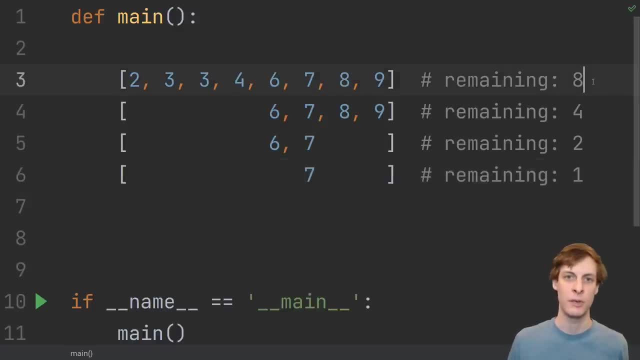 of algorithms and big O notation. Here you can see we started with eight elements and at each step we ruled out half of them. This idea of ruling out half of all the possibilities at each step is where binary search or bisection search gets its name. This is also where it gets its. 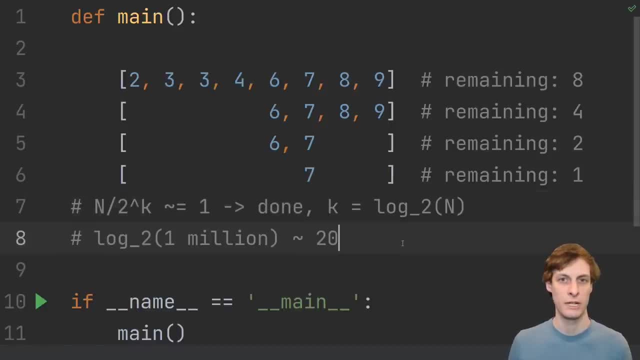 logarithmic time complexity from. So binary search is useful, fundamental and simple, And yet a huge percentage of programmers, even professional programmers, struggle to write binary search. How can the idea be so simple but the implementation be so difficult? Well, it's not so difficult, You just have to think about it in the right way. The first thing: 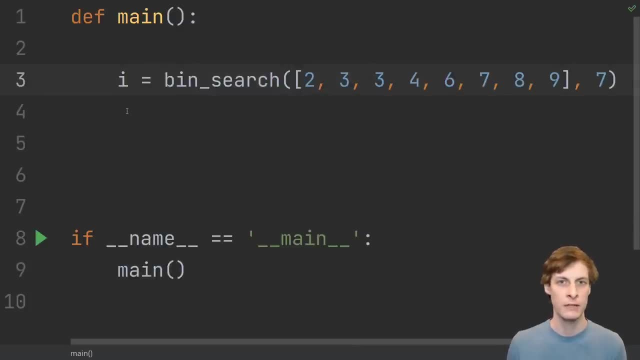 we should decide on is: are we returning the object that we find or the index that it was at? The index itself is a more useful piece of information. We can always just grab the object at that index later. But what do we do if the object we're looking for isn't there? Do we do? 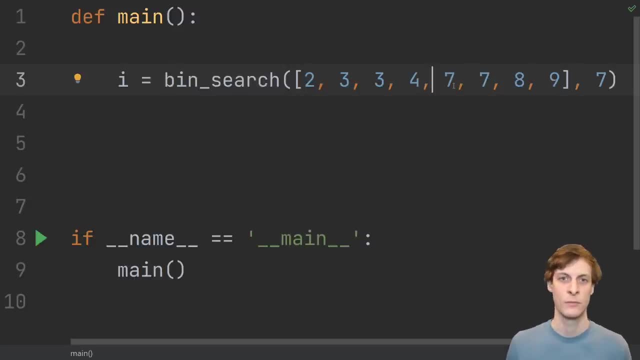 something like return negative 1 or maybe raise an exception? Or what if there are multiple valid indices to choose from? With every arbitrary choice that we make, we would have to remember the implementation details that go with that choice. A better way to do it is to rephrase the 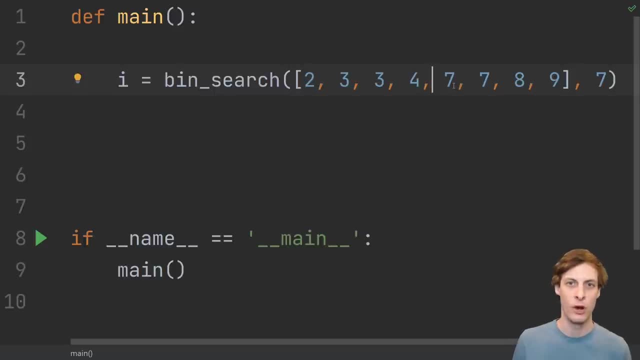 question so that there's always exactly one answer. So here's how I would rephrase the question. If I were going to add another 7 into this sorted array, where should I put it so that it's the first 7?? Notice that. 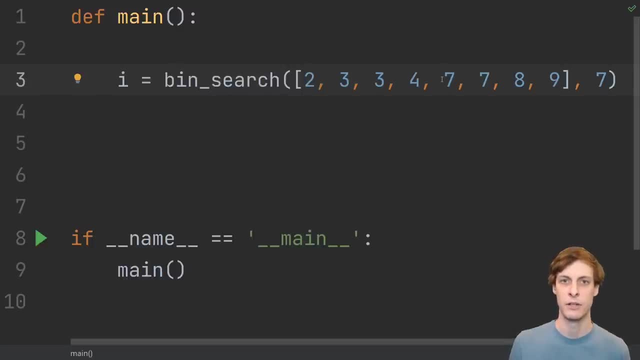 in this hypothetical, I'm always adding the 7 into the array. That guarantees the array is non-empty and always contains at least one 7.. But if it contains at least one 7, then there is always a unique first 7.. The index of that first 7 is the answer to my question. It doesn't matter. 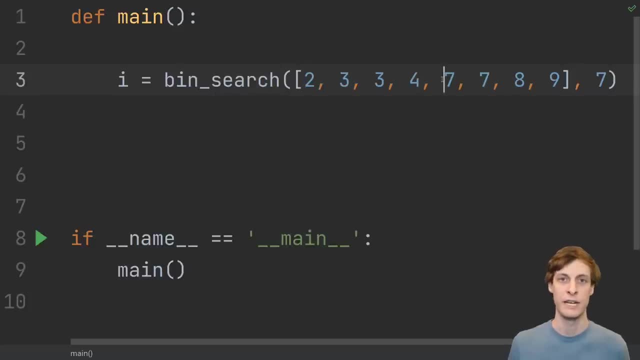 whether or not the original array had a 7 or multiple 7s in it, The location of the first 7 in the new array is always uniquely determined. If there were no 7s, I would have to put it here to maintain the sorting property, And if there are already 7s, it would have to be the index of. 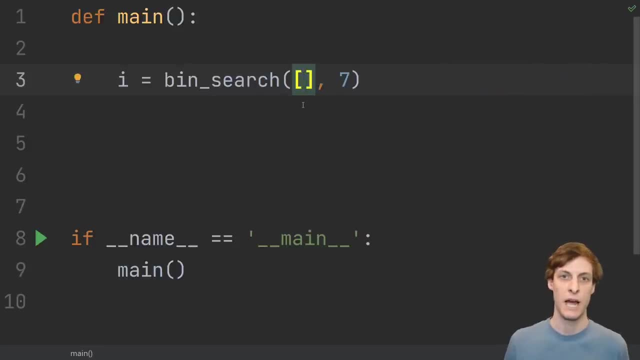 the first already existing one. Even if the array were empty, I still get a valid answer. In this case, I would have to insert the 7 at index 0.. Notice that 0 is not a valid index into this array, but it still makes sense. 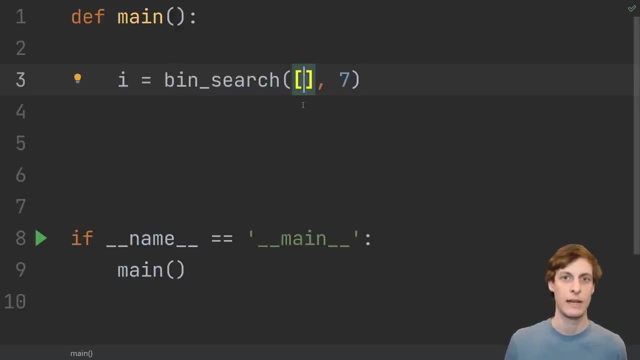 Because the question that I asked was: where should I insert it? And it certainly makes sense to insert it at index 0.. The same applies for a non-empty array. Binary search might tell me that I have to put it at the end. As long as you keep in mind this interpretation of what binary search? 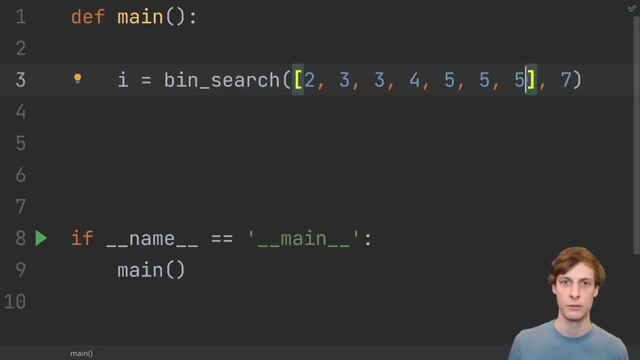 is supposed to return, it's much harder to get confused. I think that far too often, binary search is taught solely as an algorithm that works on sorted arrays, But the array being sorted, I claim, is not actually a sorted array. It's actually the property that we're using here Here. look, I changed some of the elements and this: 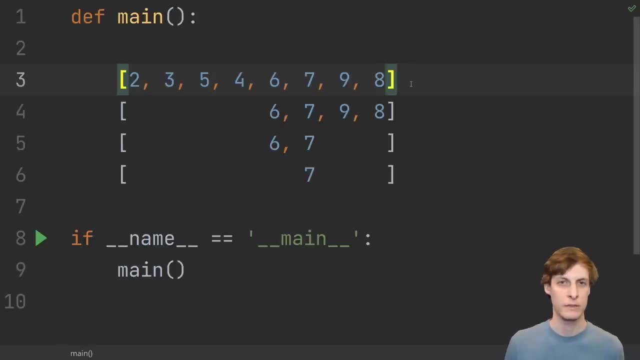 array is no longer in sorted order, But notice, the steps are exactly the same. What we need is that everything less than 7 is on the left and everything bigger than 7 is on the right. In this array, the numbers have been replaced with the important information. Is this number less than? 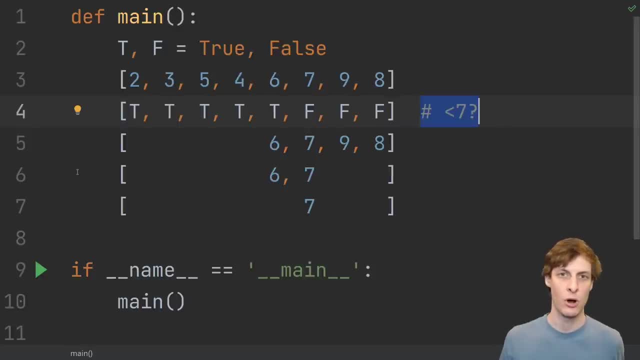 7?. Notice how any trues are on the left and any falses are on the right. So, now that we're looking at the relevant data, where do we insert 7 so that it is the first 7?? Notice that the answer. 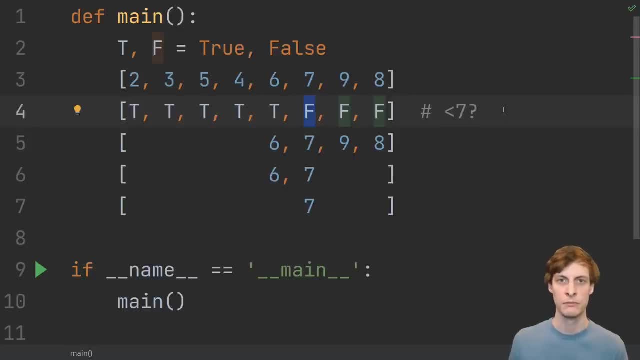 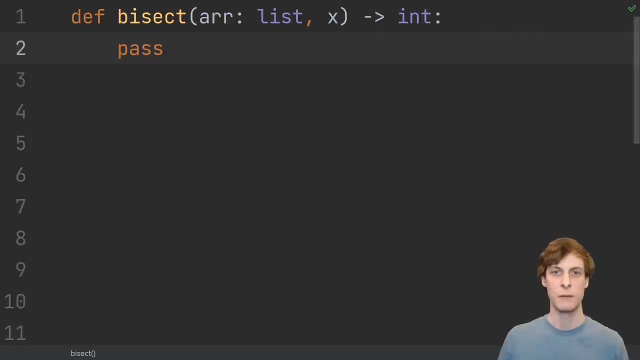 that we're looking for is the index of the first false value, or the end of the array if there are no false values. This is the key insight that we need to keep in mind. that makes the implementation extremely easy to remember. Squint your eyes and find the first false value. Okay, let's write the 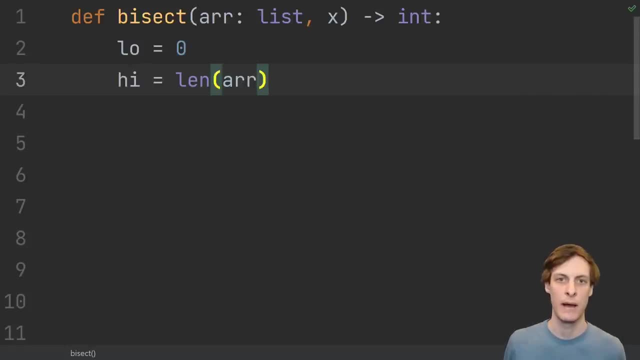 implementation. Low and high are lower and upper bounds on where this first false index is. Zero would mean the first value is false and length of the array would mean that all of the values are true, so we would need to put x at the end. The idea is that we are. 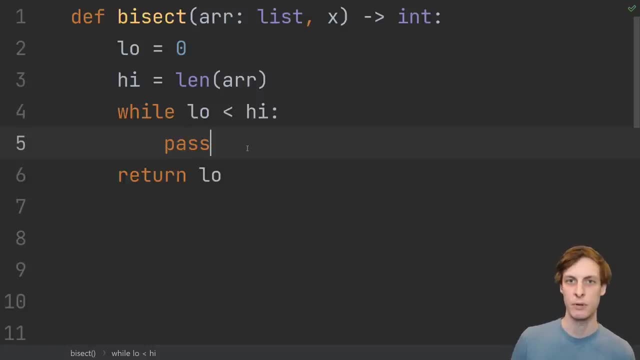 going to continually increase our lower bound and decrease our upper bound. until they're equal, Low and high will meet at the unique index that we're looking for, so we could return either low or high, It makes no difference. We compute mid, which is the closest index to the middle, between. 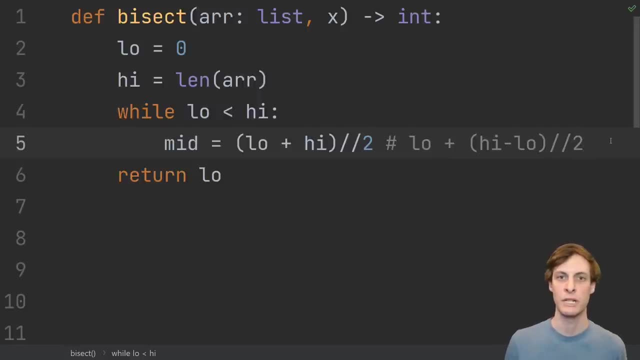 low and high. Python can represent arbitrarily large integers, so we don't need to worry about overflow. But if you're doing this in another language besides Python, you might have to worry about overflow. In that case you can represent the midpoint equivalently by writing it as low plus half the distance between low and high. 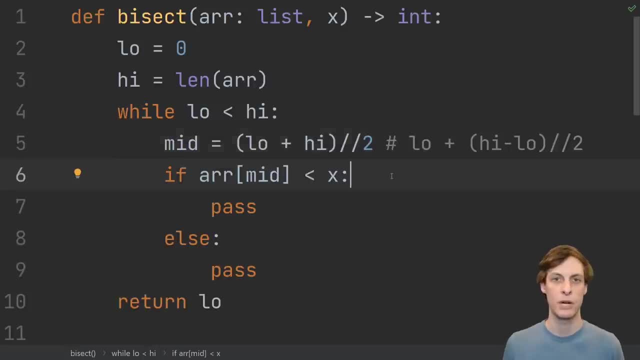 If you write it this way, it will never overflow. Next comes the part of the algorithm that is most often written incorrectly. We need to compare whatever's in the array at the midpoint with our given x and then update the lower or upper bound accordingly. Remember. 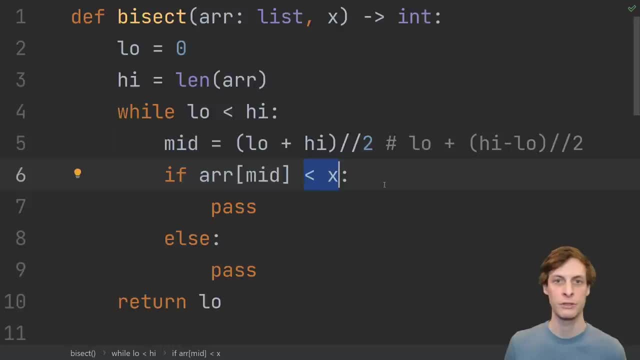 we're looking for the first false value, where true or false is determined by asking the question: is this less than x? Well, in this section, the middle value is less than x. It is a true value. Since the value at mid is a true value, the earliest a false value could occur. 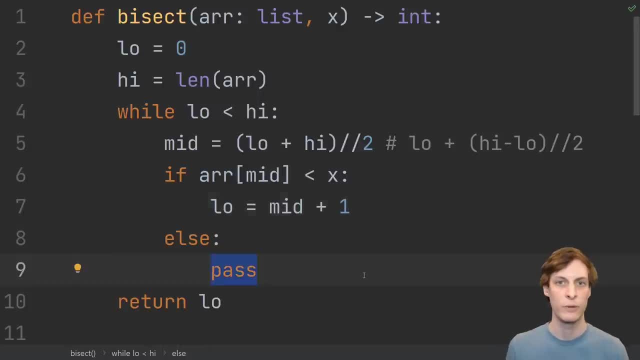 is the next one, which is mid plus 1.. What about if we see a false value? In this case, the first false value couldn't be any later than mid, because there is a false value at mid, but it could be another false value before the one that we've found. That means the best we can do is update. 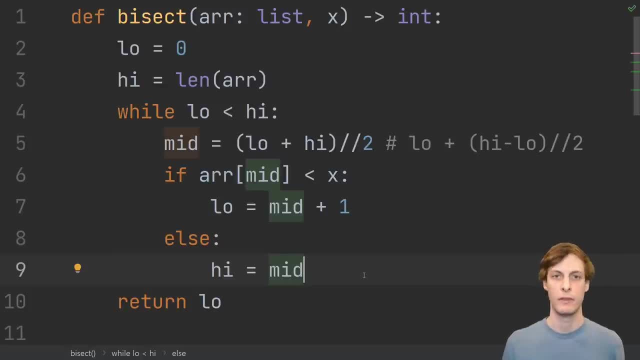 our upper bound to be whatever mid is. And there you have it. This is a correct implementation. But how can we reason about it? How do we know that this actually gives the right answer? Well, we know that low is always less than or equal to. the correct answer is always less than. 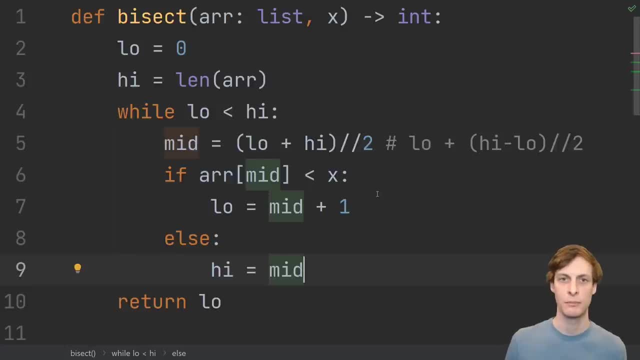 or equal to high, and we do keep updating the lower and higher bounds, but how do we know that they actually meet so that the loop stops? It's enough to show that every iteration the difference in low always decreases by at least 1.. If we enter this clause, the plus 1 ensures that low. 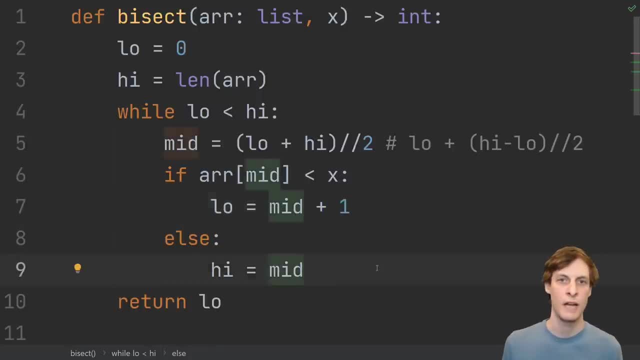 always increases by at least 1.. In this clause we're setting high to mid, so hopefully we're lowering high. but how do we know that mid was actually strictly less than high? Here we're actually using that integer division rounds down Inside the while loop. low is less than high, so 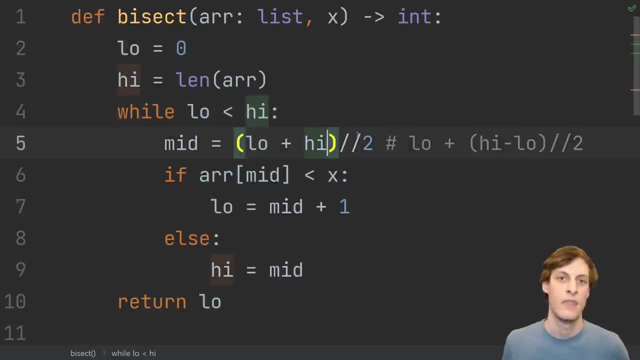 low plus high is strictly less than high plus high. That means that when we divide by 2 and round down, we'll get something strictly less than high. So we're actually using that integer division rounds down Inside the while loop. low is less than high, so low plus high is strictly less than high. 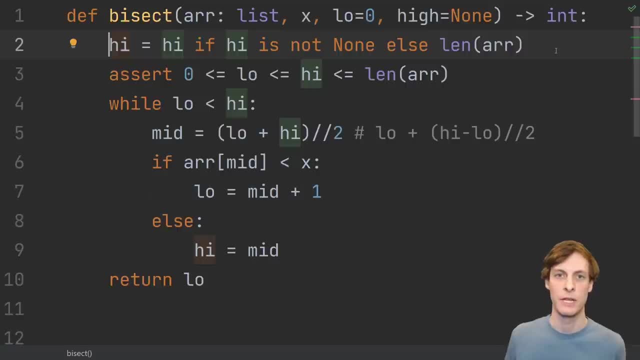 It's common to take low and high as optional parameters, so that if you already have a lower or upper bound, you can make use of that. And, of course, don't forget to check that the parameters are valid. And that's all there is to it. But wait, you ask instead of returning the index. 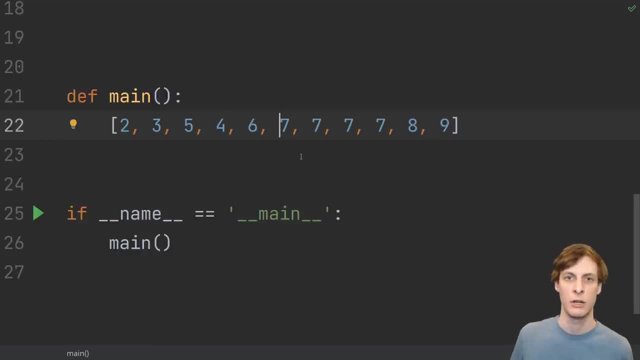 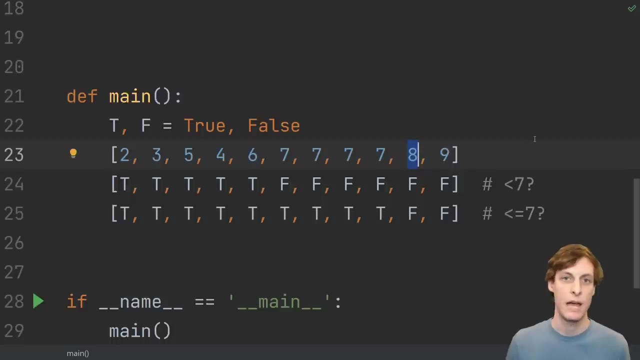 to insert a 7 so that it would be the first 7,. couldn't I also return the index so that it would be the last 7?? Yeah, you could. You could follow essentially the same analysis and get a very similar algorithm To find where it should go. to be the first 7,, you'd have to go to the first 7,. 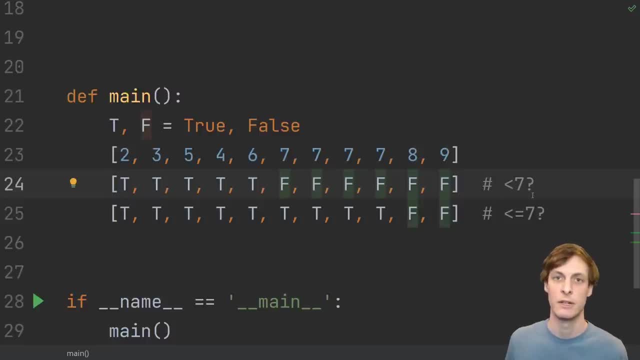 the relevant piece of information is: is it strictly less than 7?? To find where it should go to be the last 7, you want to know: is it less than or equal to 7?? In either case, the index that you're looking for is the first false value. You just need to decide on what you. 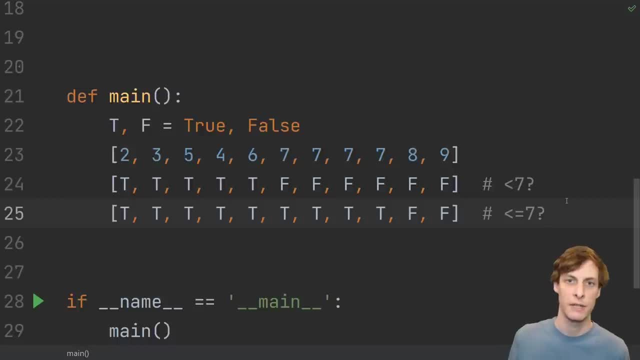 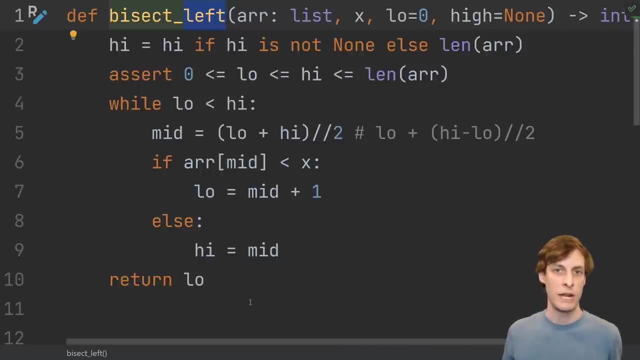 mean by true and false. The first one is called bisect left and the second bisect right, So this one that we already wrote is bisect left. Can you tell me what you need to change in order to make it bisect right? Here's an example of how you might use bisect left. 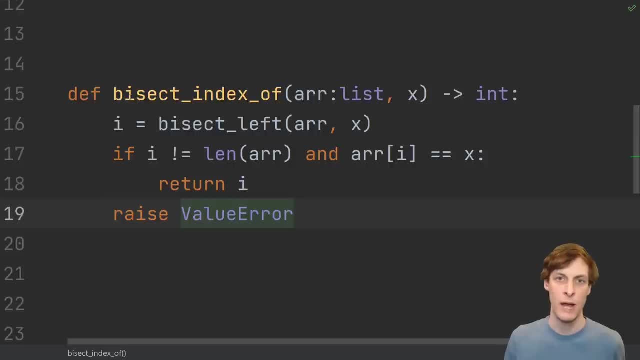 For this function. we want to find the index of the first x in the array, or throw an error if there isn't one. Since we're looking for the first index, we'll use bisect left. If there is already an x in the array, bisect left will return the index of the first one. 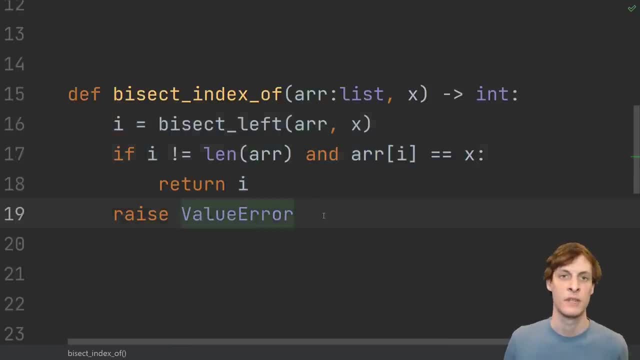 So we would like to just check at that index and see if we see an x, If we don't get back a valid index or if we find that there is not an x at the location that bisect left told us to look at.